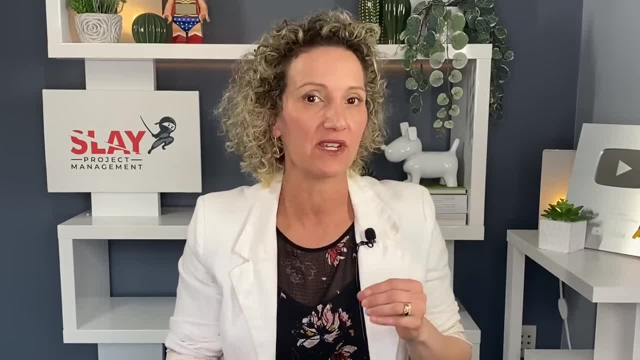 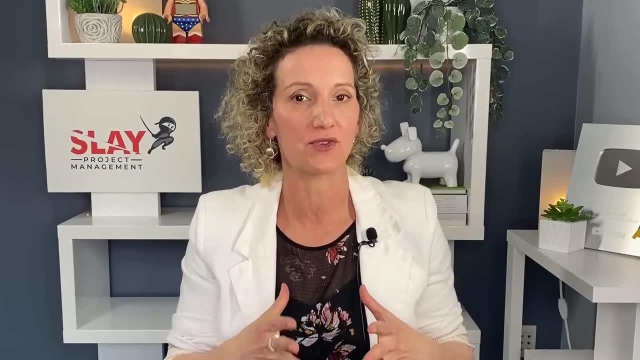 because it's the detail. The devil is in the detail. So if I have an understanding what's in scope and what I'm not doing, which is out of scope, then that allows me to start brainstorming and understanding how much am I going to really need to make this deliverable? 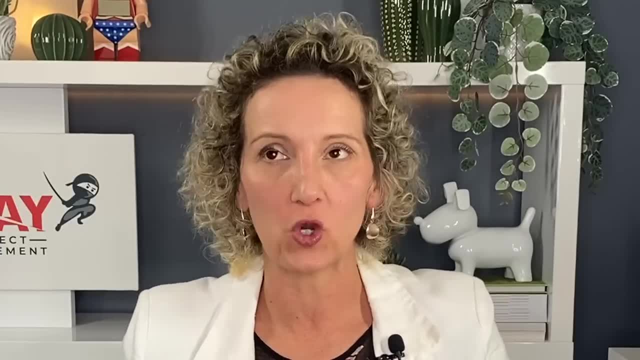 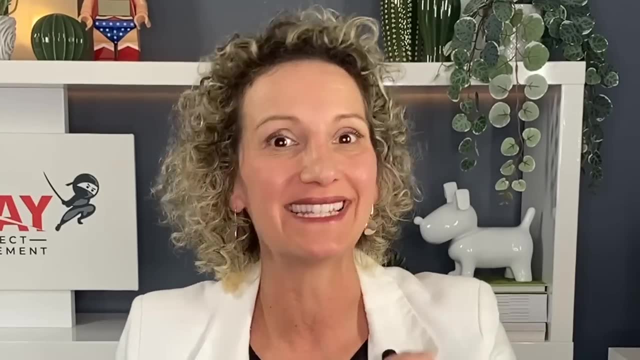 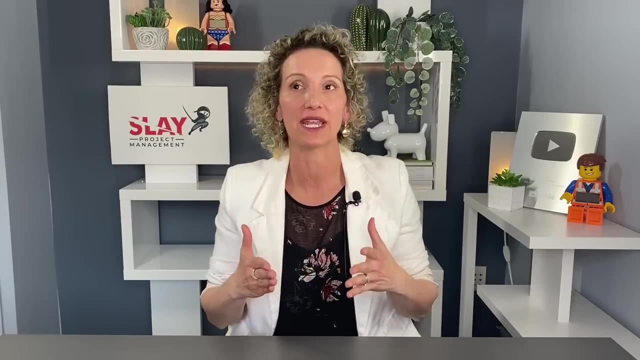 come to fruition. So that scope statement absolutely huge, something that's important. You need to get that locked down And you need to get it approved. Once you get it approved, then you can start asking for the budgeting around that and figuring out how much are things going to cost to actually make this. 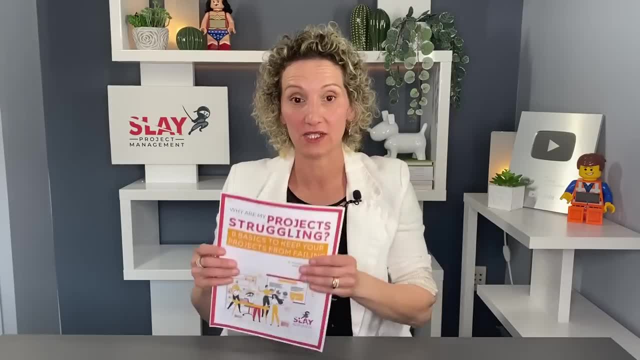 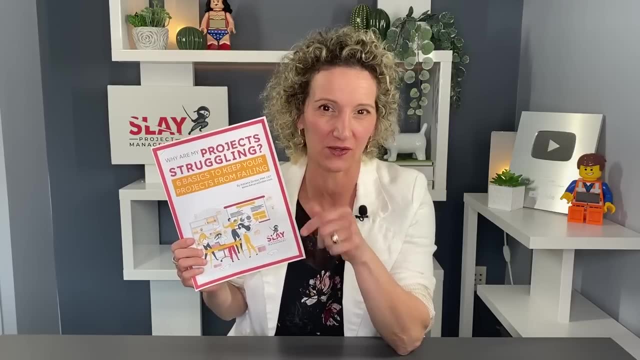 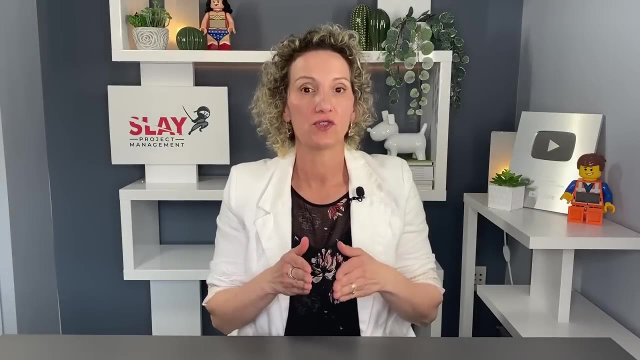 scope come to fruition. Okay, before we continue, see this here. If you're going to do budgets, you're going to need this. I'm going to tell you later on in this video how you can get your hands on it, So stay tuned. Step two: you need to identify direct cost and indirect cost. So, in order to do 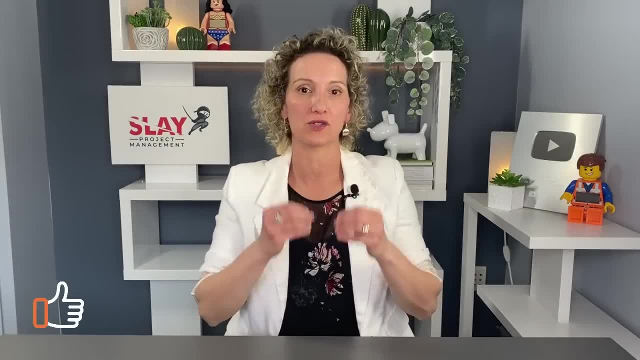 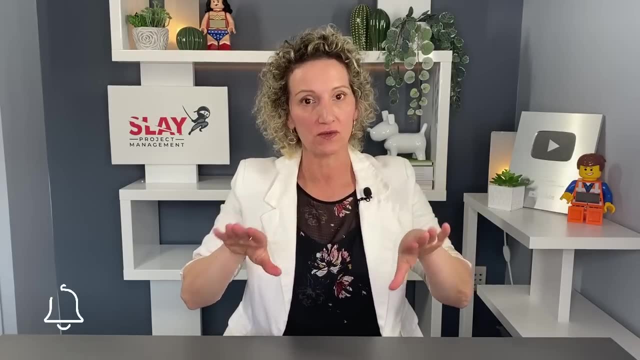 this you have to do step one. You've got to be really clear on your scope and everything that you're going to be delivering and really spend time figuring out what that is, Because now you have to bucket it into different areas. You have your direct costs, which are costs that are 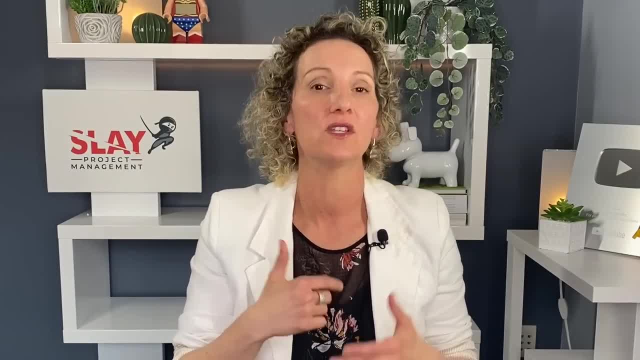 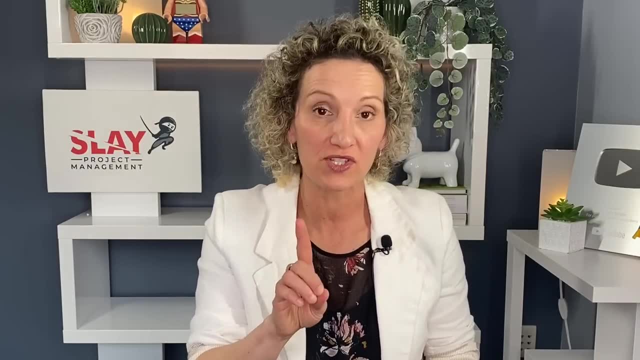 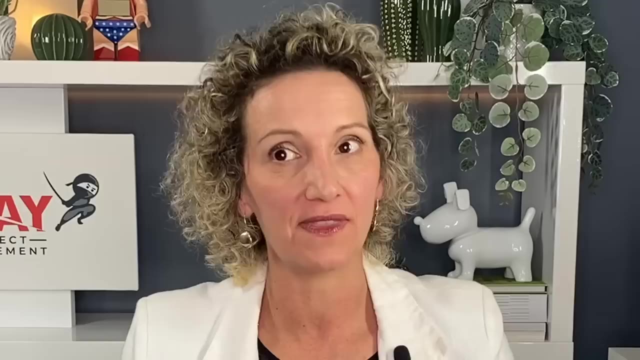 directly related to what you're doing. They're usually one-time costs, So if you're installing new hardware somewhere, you've got to purchase that hardware. You're only going to purchase it once. You also have to think about that. These are subsequent costs. These are costs that can be. 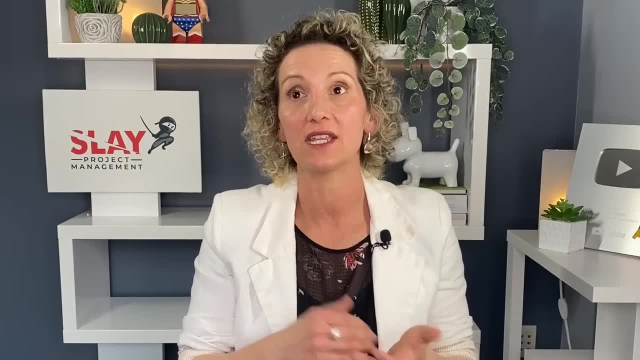 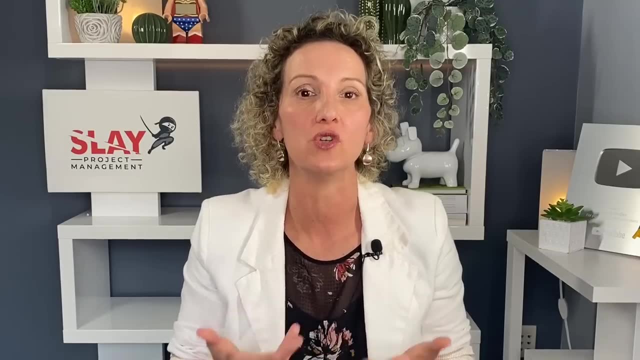 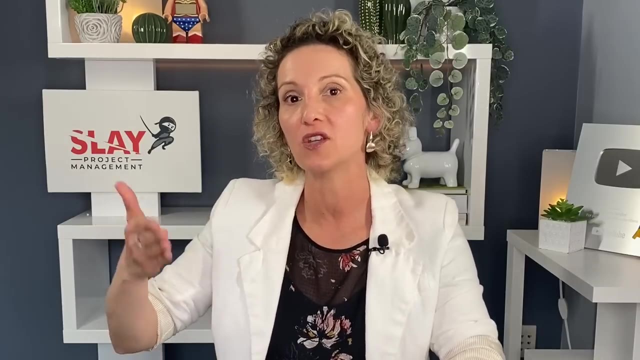 repeated. So in that same example, let's say you have software that's going to go on that hardware and it's a software license that you purchased that has to be renewed every year. That's now an indirect cost to the project. Yes, you're going to purchase it once, but now, every year you have. 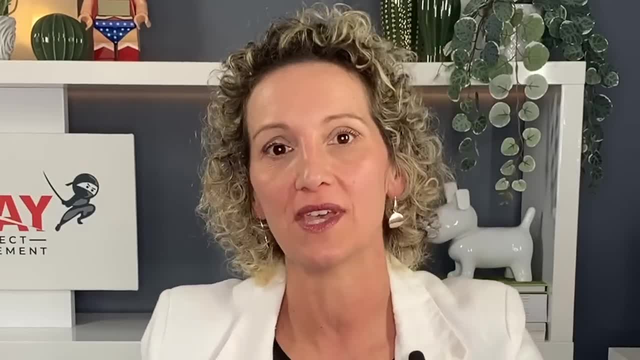 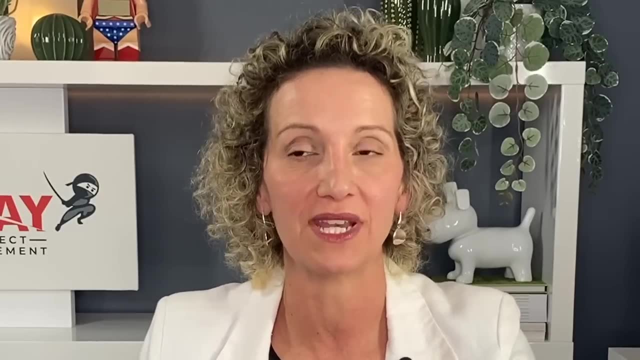 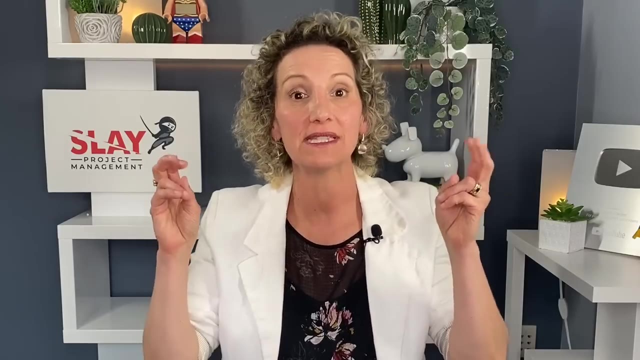 to renew it. Now who's going to maintain that? So that's the indirect cost. Why do you have to do that? Because your budget will cover the direct costs, but it's not going to cover the continuous indirect costs. You have to pass that off to what we like to say: the business, The business. 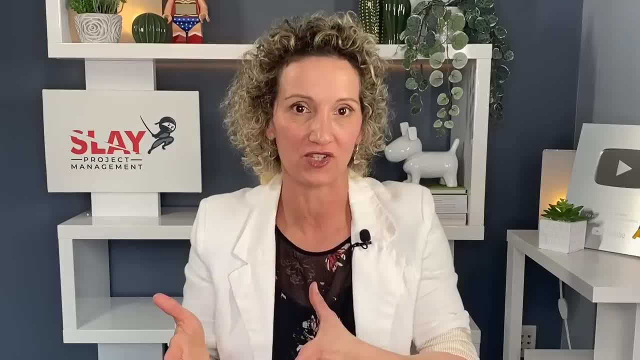 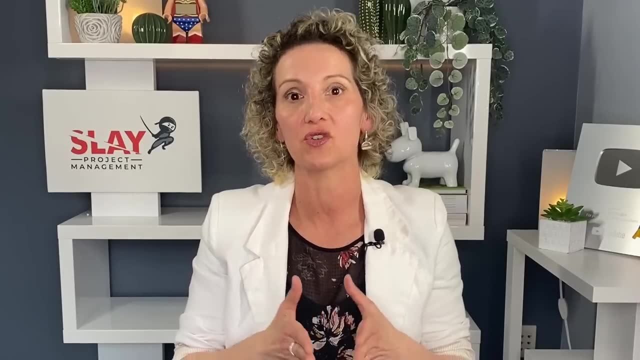 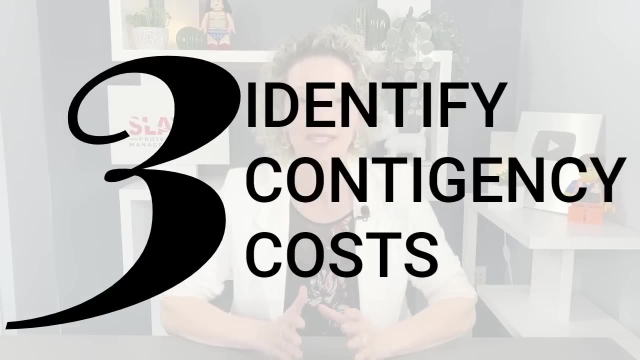 is going to be taking it over. They now have to add that to their budget. So you've got to understand those things, because now you're going to have to negotiate and bring those people on board and ensure everyone's on that same page. So that's really step two, Step three: identify: 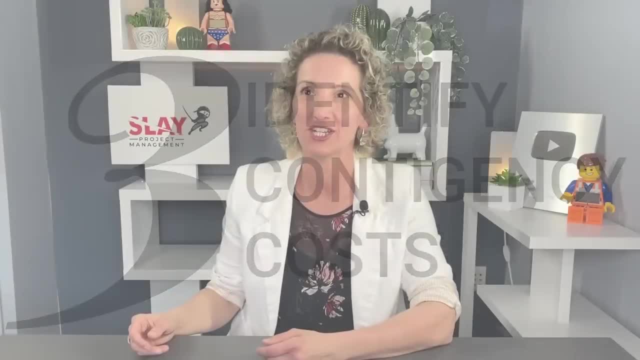 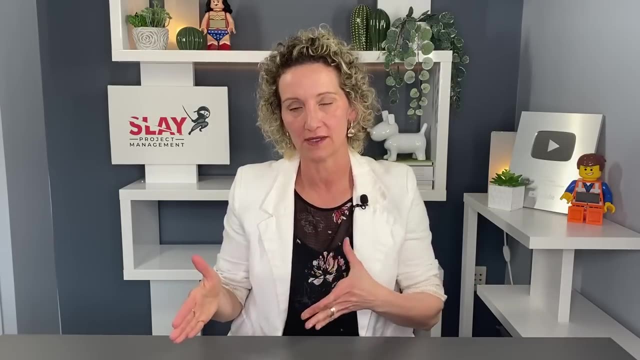 conditions. What is contingency costs, Adriana? why are there so many costs? Well, because you're dealing with budget. I promise you there's tons of things to think about. So what is contingency costs? These are things that pop up in the project that you couldn't plan out. Maybe they're associated. 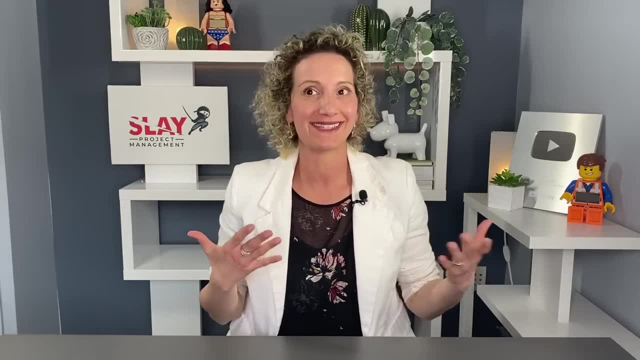 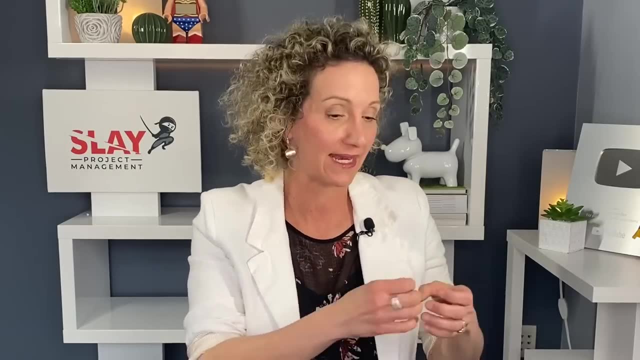 with risk and the risk came to fruition, or they're just things that, as I said, you couldn't plan out, you didn't even think about, So you kind of have to have- I call it- banked hours or a bank of money for contingency things. 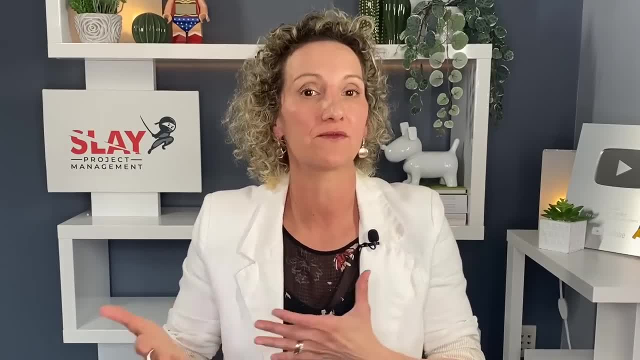 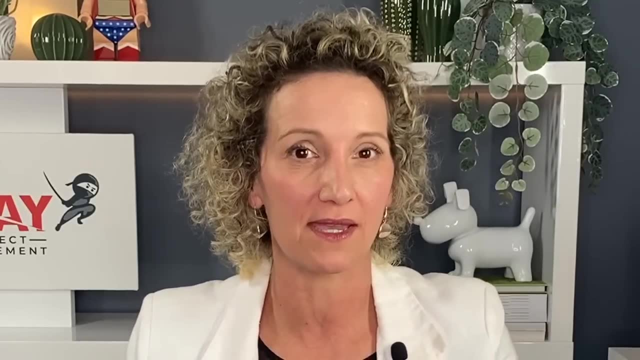 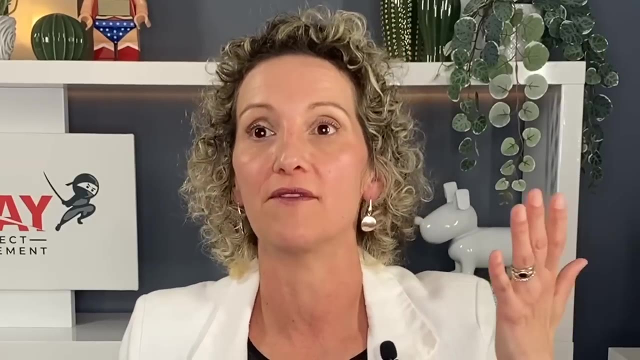 That you need to ensure, get covered, to make sure your project comes to fruition. So a lot of times you can pre-plan those things in a way by thinking of, for example, you purchased hardware, it's coming from another country, You have to ship it and you have custom. costs associated with it And if something goes wrong with that shipment and you're, let's say, you need to expedite it for whatever reason, because the manufacturing was later than expected. So now you have to make sure that everything is okay, Air freighted over versus doing it on a ship. leaving me two different costs. So you want to have those contingency costs in place in case you need to act on your contingency plan. So that again is something else you have to think about and build into your budget. Don't get me wrong: You don't have to plan for every contingency, but you do. 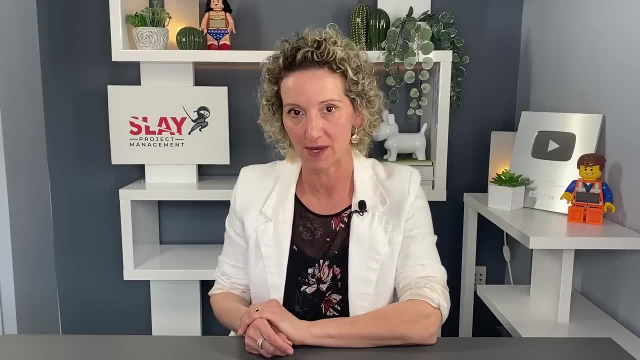 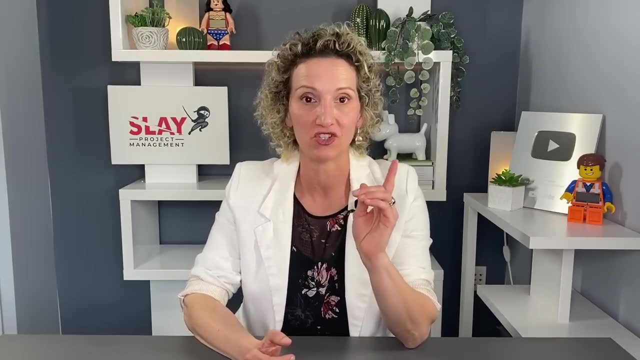 have to have some sort of bank contingency budget to cover those types of things that may pop up. Okay, All right. So, okay, Okay, directly related to budget, I just mentioned it about risk. You need to know how to do risk. 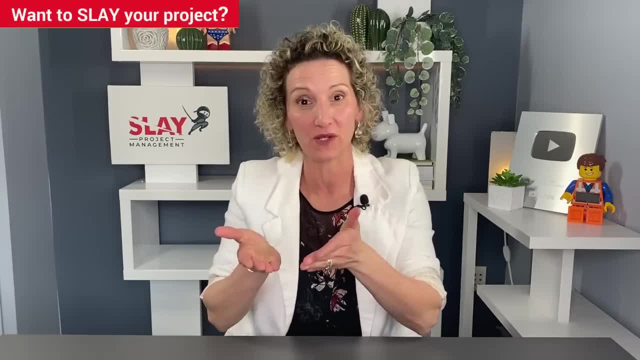 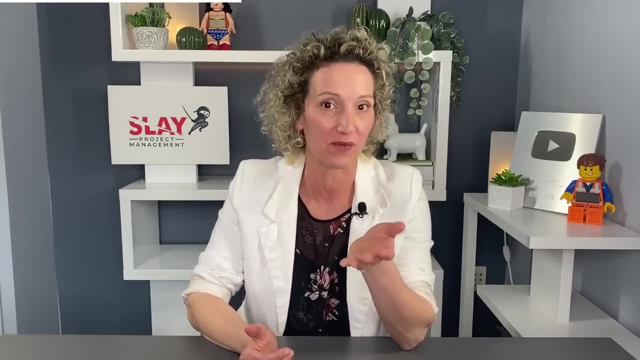 planning as well, because through your risk planning that's going to bring up the contingency that you need And, as my SLAY students say all the time, they're so grateful for the risk mitigation and contingency planning that I have in the course, If you're interested in it at all. 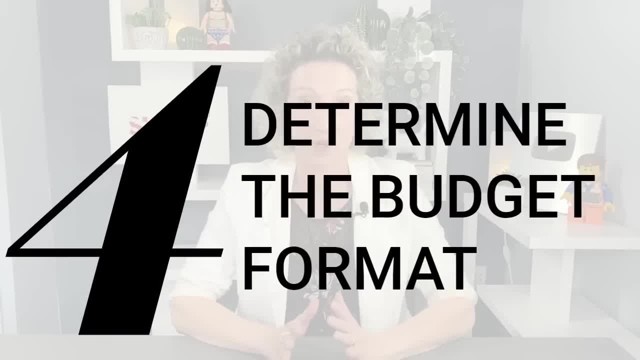 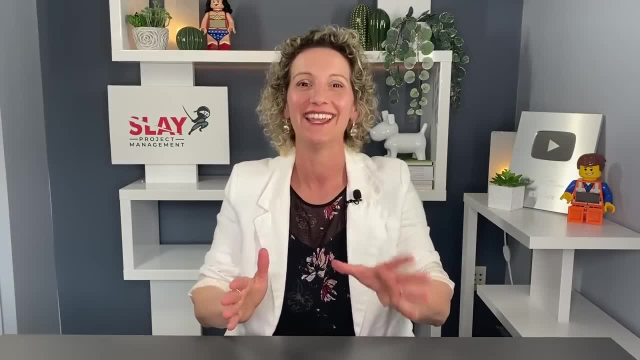 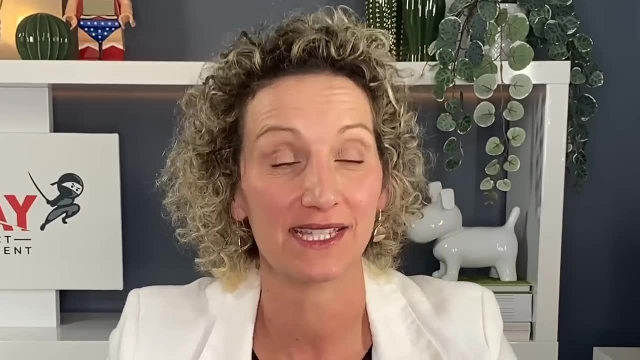 go check it out. It's in the link below. Step four: determine your budget format. Okay, so now you have step one, two and three all locked down. That's your job as a project manager. Now what you need to do is: don't guess the format. go to a finance person, because I promise you. 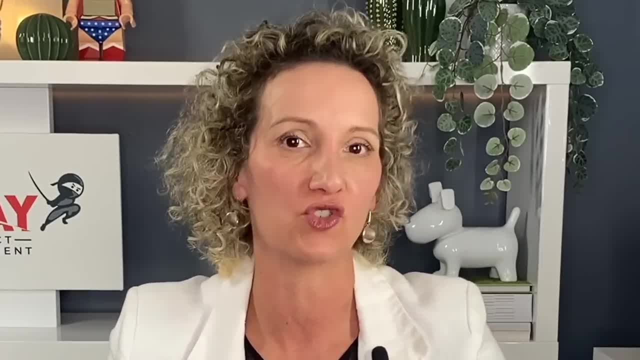 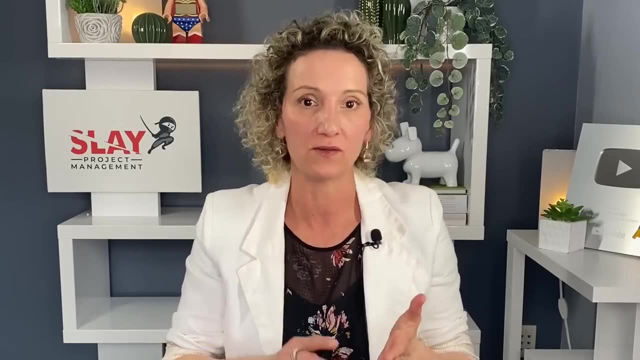 if you're dealing with a big budget, finance has a way that they want you to track it. They probably have specific spreadsheets that they want you to use because it makes it easier for them. So connect with senior executives, connect with your sponsor and connect with a finance person. 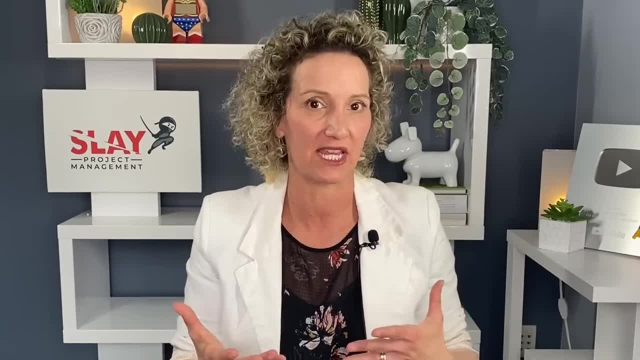 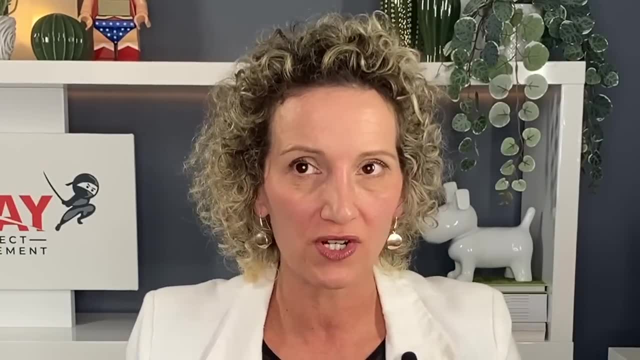 to find out. how do they want you to track it? They may even have a way to track it, but they don't have an expectation on reporting on that budget. So, again, if there's not a clear cut reporting structure, I think the bare minimum is: here's what I have. here's what I've spent. 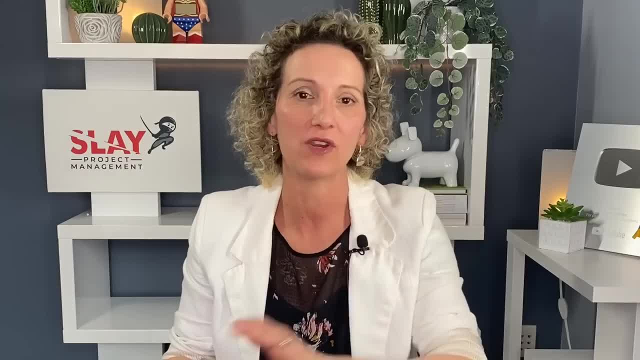 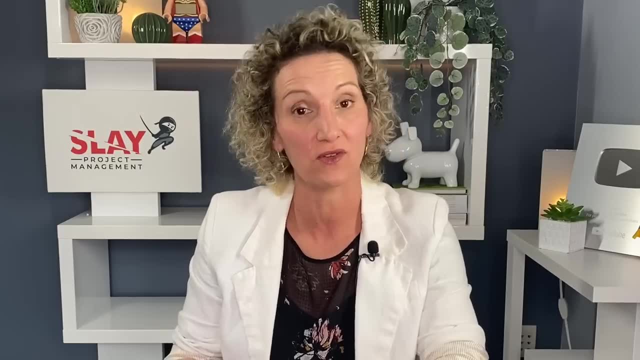 here's what I have left over. That's the bare minimum. Again, every organization is different. It is your job to check in with the finance department to figure out how do they want you reporting on this budget so that you can follow their format. Step five: allocate budget to. 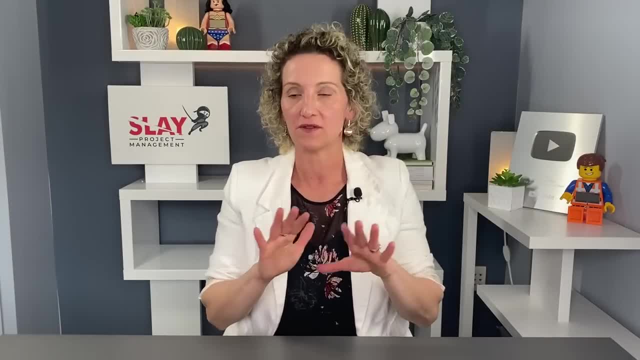 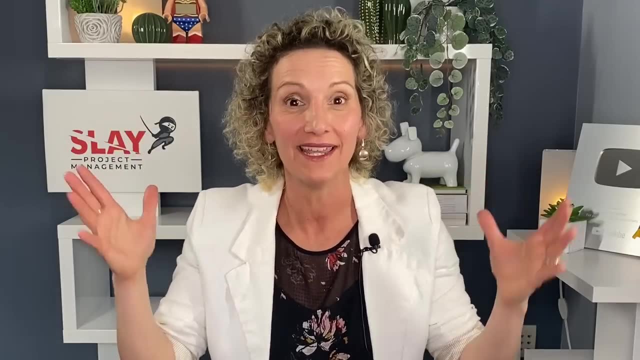 tasks or activities. So now that you have your budget, you're very clear. you now have to allocate that, So you need to have an understanding that it's not just one big pot of money. It is certain parts of that money is going to go towards certain things, So you need 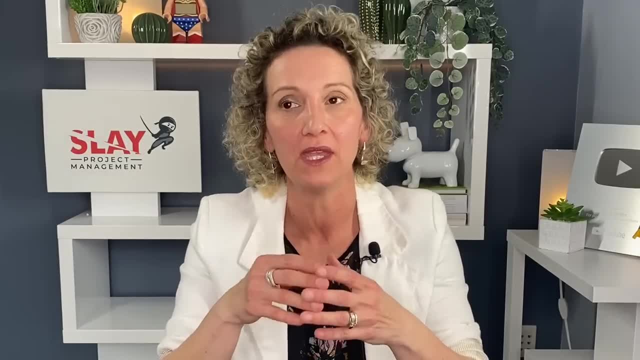 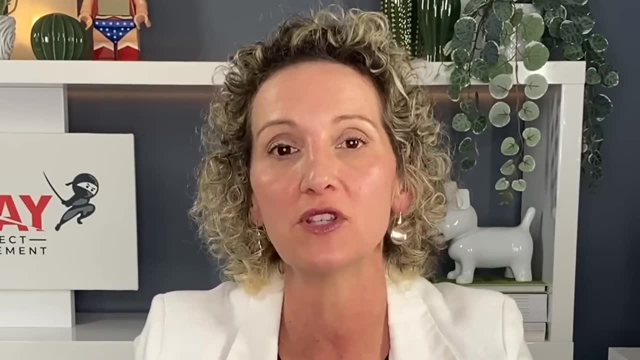 to allocate it so that you can keep that under control. It's really important so you don't overspend in one area and then impact another area. You have to know how much money do you have to spend, For example, on training material. let's say you're. 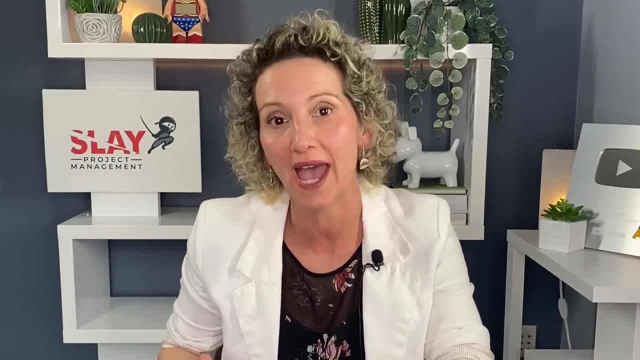 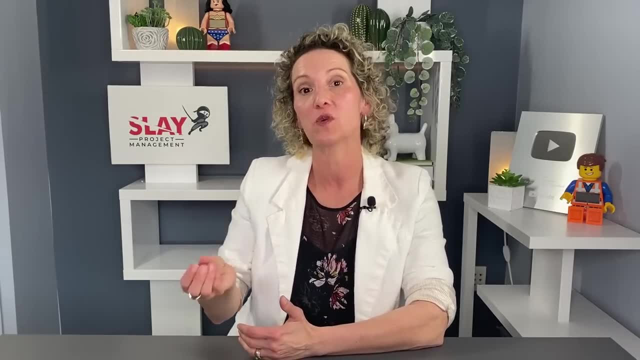 executing a new software and you have to create trading material. Well, how much money do you have for that? That's going to dictate the type of material you use, the type of training you're going to have. That's why budget is so important, because it gives you your parameters on what 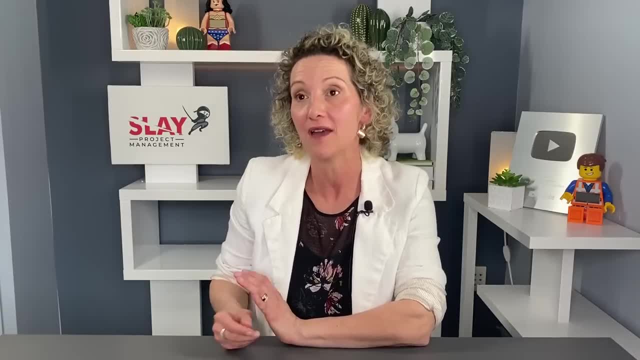 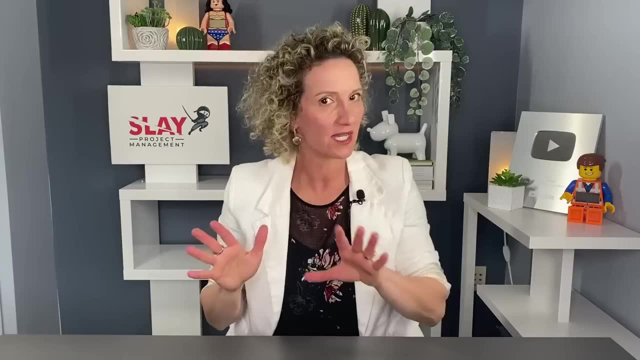 you're going to do from a task and activity perspective, because you only have X amount of money to spend. Step six: monitor and manage the budget. Okay, We touched upon this because I said: find out the spreadsheet from the finance person because you have to report into them and 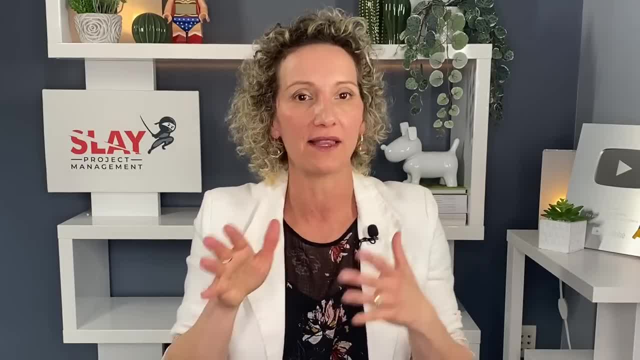 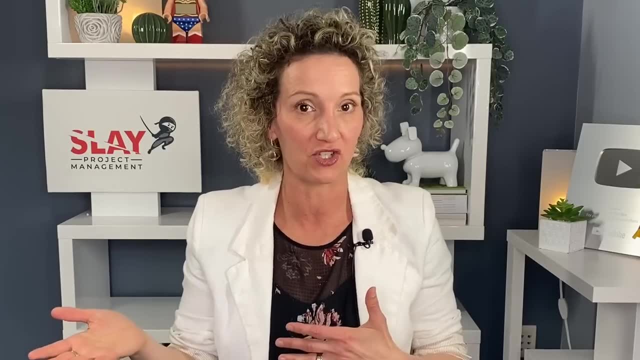 give them what they want. This is why- because now that you've allocated everything, you're very clear: you have your money. you have to monitor it. You're going to need to have your team members if they're spending some of that budget because, again, as the project manager, you're going to 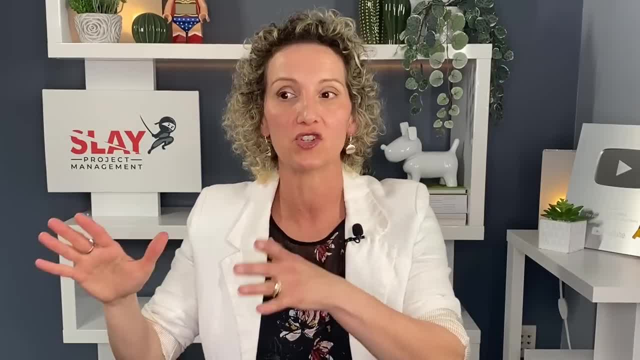 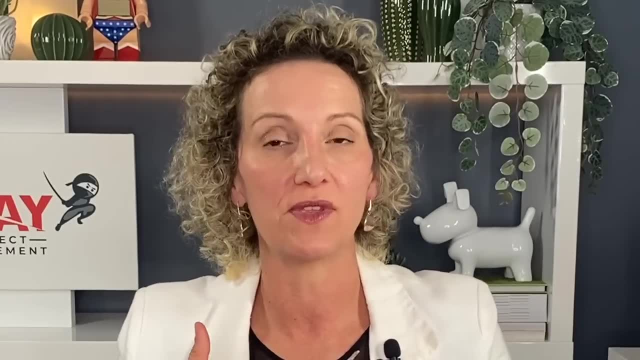 have hardware engineers. You're going to have individuals who are in charge of purchasing certain stuff. You just need to ensure that they come through you. They give you the invoicing they share with you, the statement of works that they're doing, et cetera, So you can monitor.